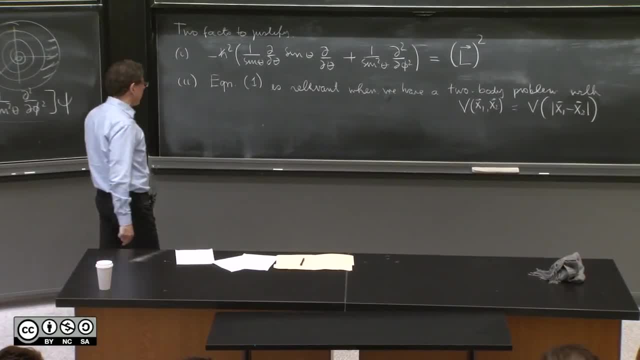 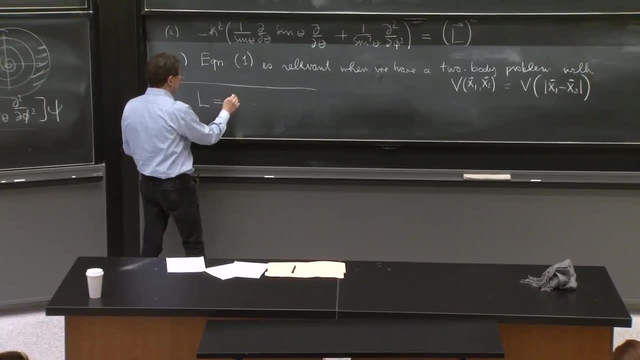 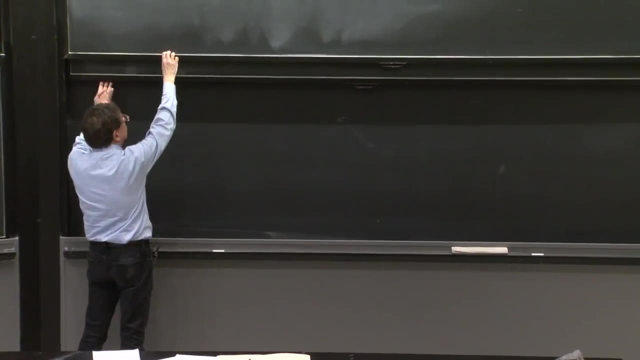 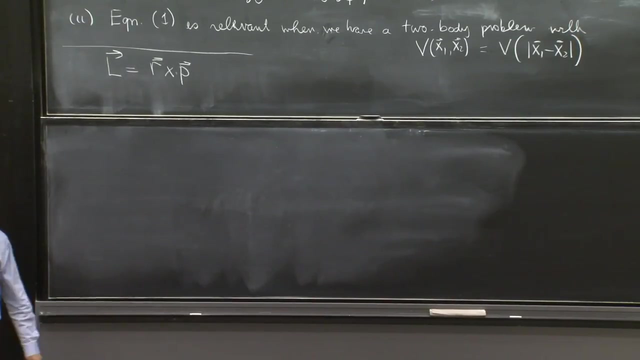 So angular momentum. we need to deal with angular momentum And the inspiration for it is classical. You have L is r, cross p classically, So let's try to just use that intuition and write the various operators And in fact we are lucky in this case. 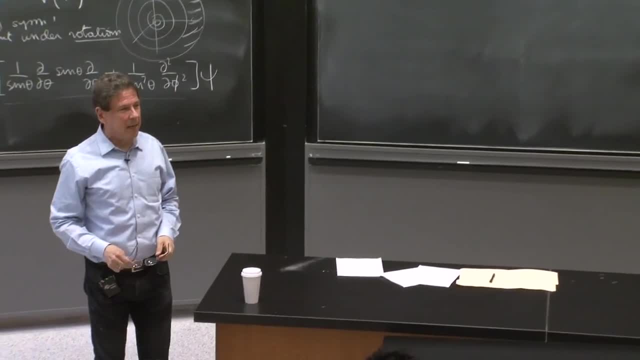 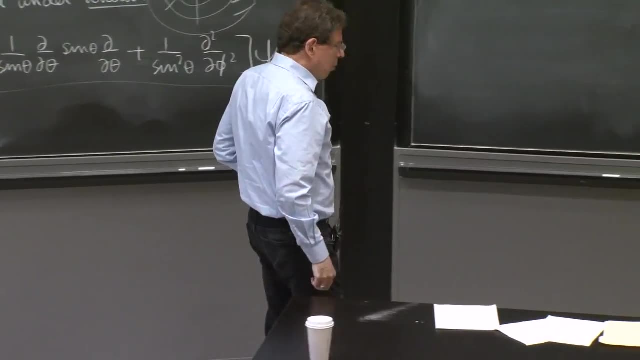 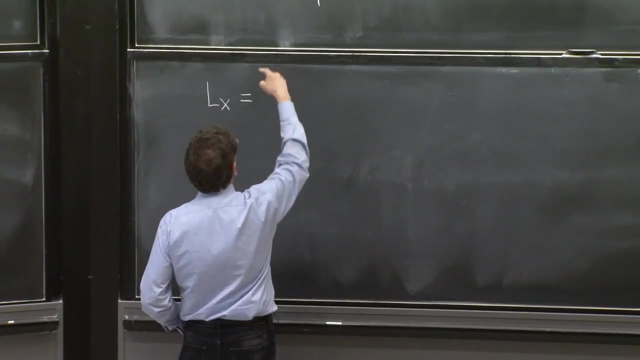 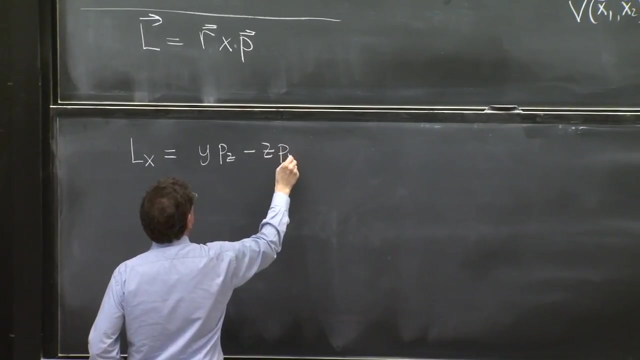 The operators that we would write, inspired by the classical definition, are good operators and will do the job. So what do we have? Lx. if you remember the cross product rule, that would be y, pz minus z, py. Now you can think of these things. 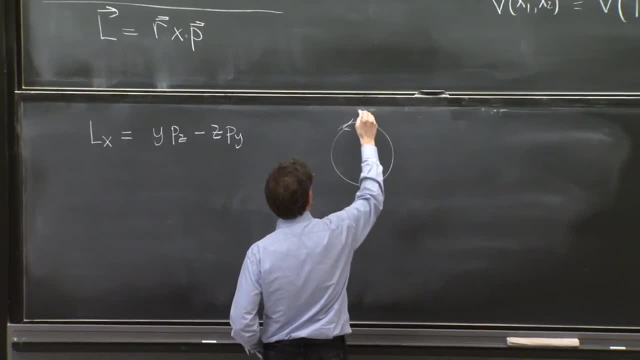 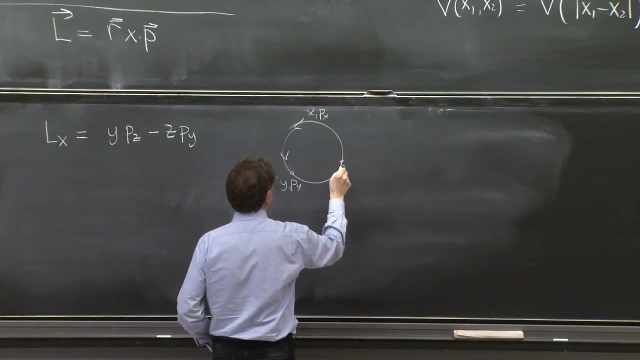 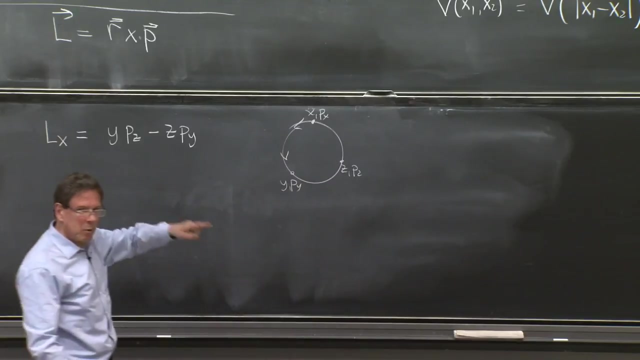 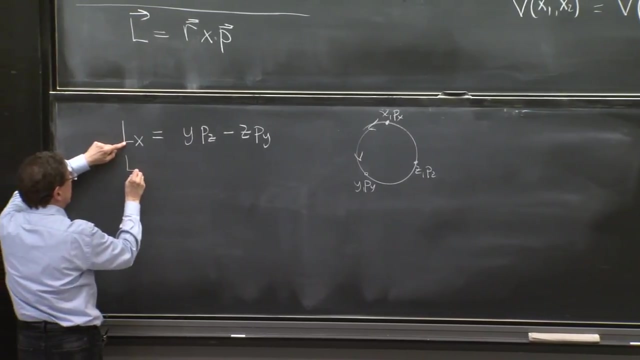 as a cycle, Like a circle in which you have x and px, y and py and z and pz. Things are cyclically symmetric, There's no real difference between these coordinates, So you can go cyclically here. So you say: let's go cyclic on this index. 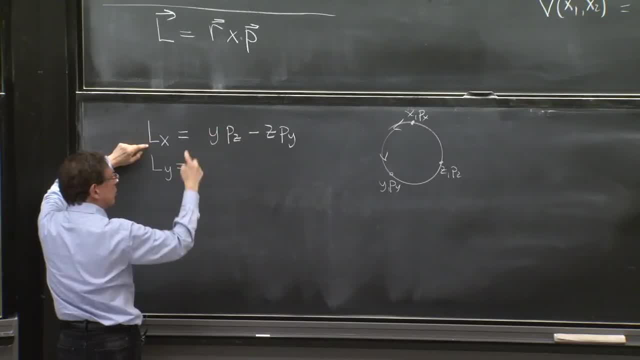 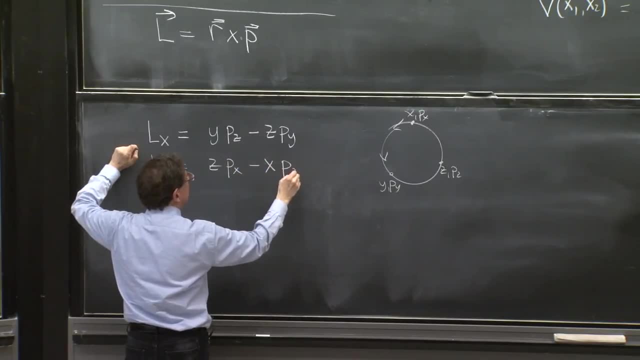 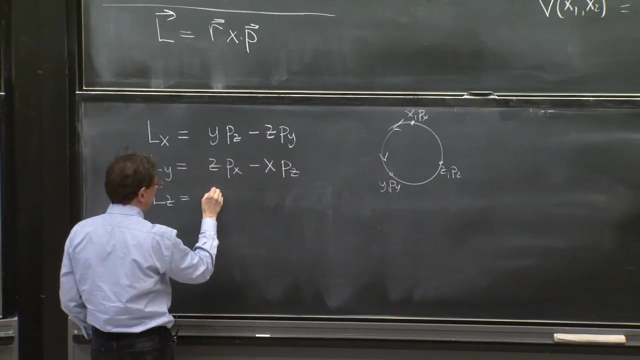 Ly is equal to the next cyclic to y in that direction is z, So that's y px minus x pz. And Lz is equal to x py minus y px. And these things I'll think of them as operators. Let's put hats to everything. 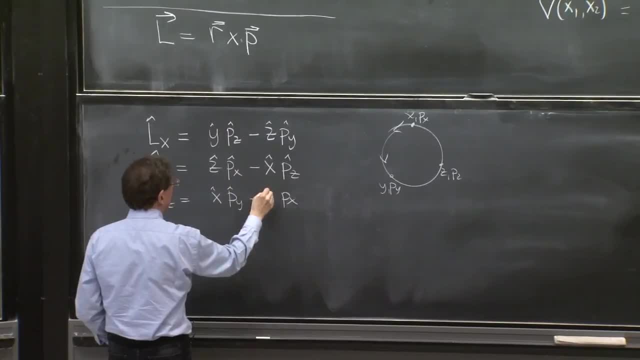 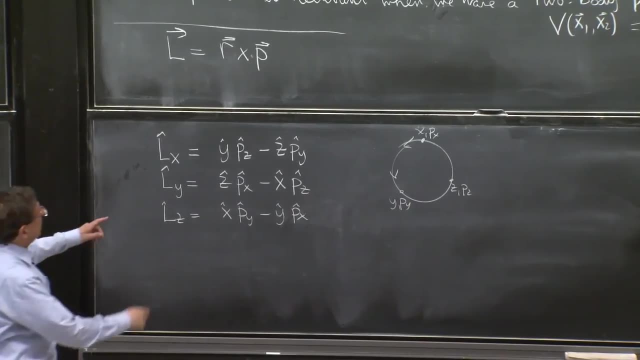 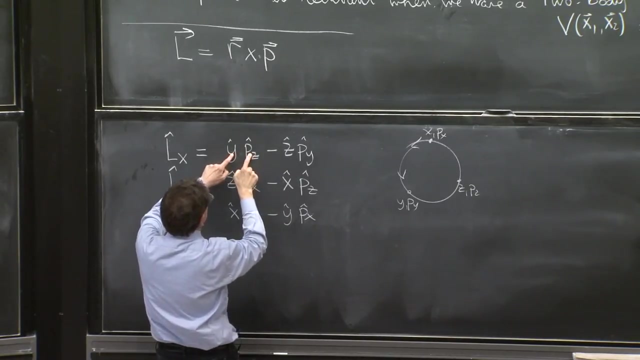 The first thing I could wonder, with a little bit of trepidation, is: maybe I got the ordering wrong. Should I have written here classically: you put r cross p and then the order of these two terms doesn't matter. Does it matter quantum mechanically? 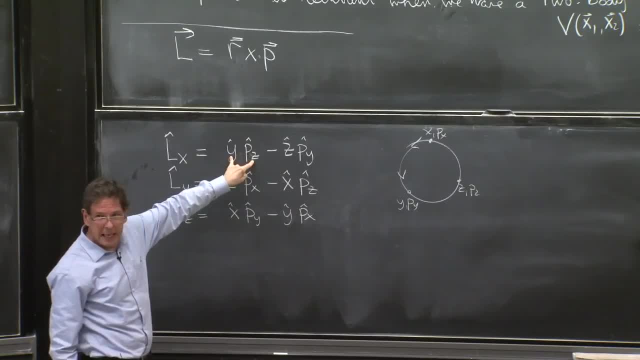 Happily, it doesn't matter, because y and pz commute, z and py commute, So you could even have written them the other way. You could have written them the other way, and they're good. All of them are unambiguous. You could have even written them the other way. 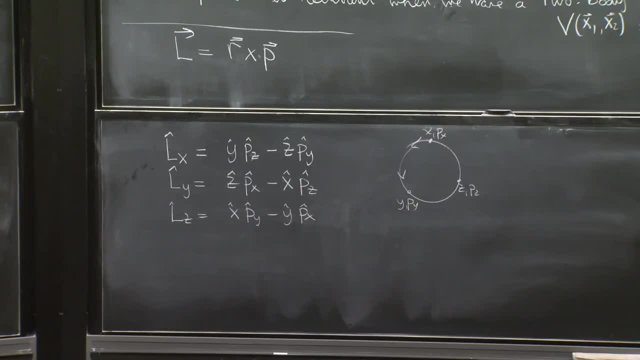 and they would be fine. But now these are operators And, moreover, they are Hermitian operators, Hermitian. Let's see Lx dagger. Well, the dagger of two operators you would do pz dagger, y hat dagger. 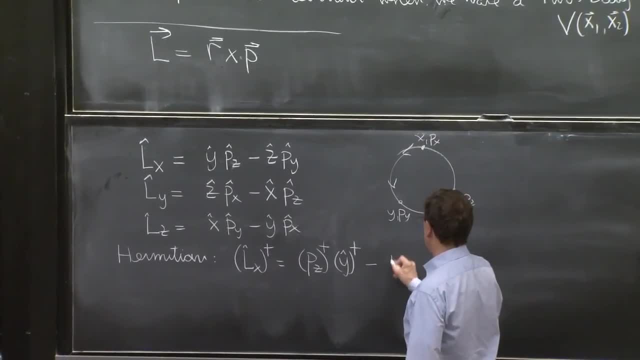 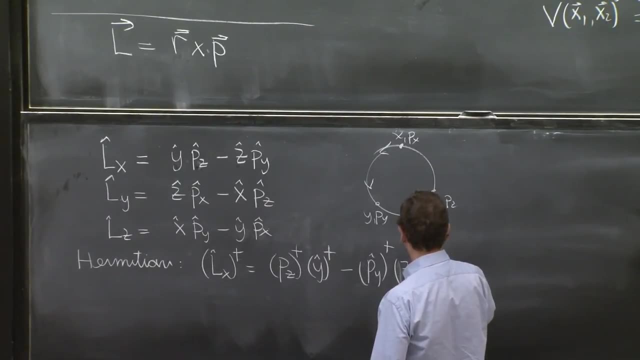 Recall: the dagger changes the order: minus py dagger, z dagger. Now p and x's are all Hermitian operators. So this is pzy minus py dagger, This is pyz, And we use again that y and pz commute and z and py commute. 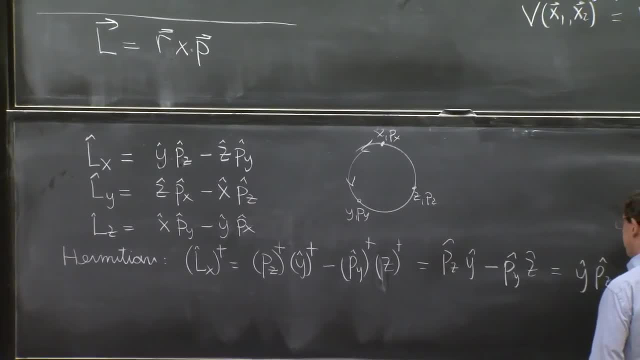 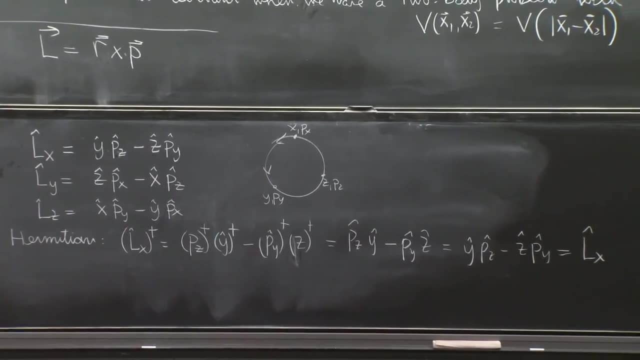 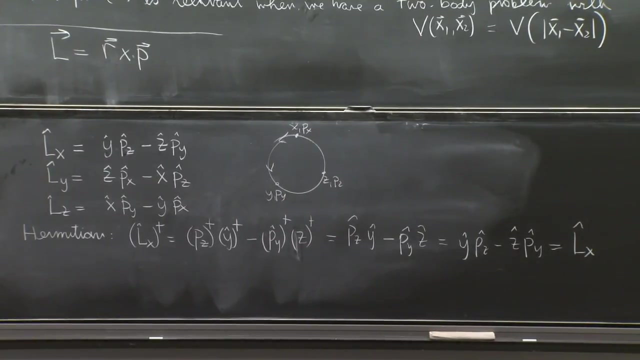 to put it back in the standard form, And that's again Lx. So it is a Hermitian operator, And so is Ly And Lz And Lz And Lz. That means these operators are observables. 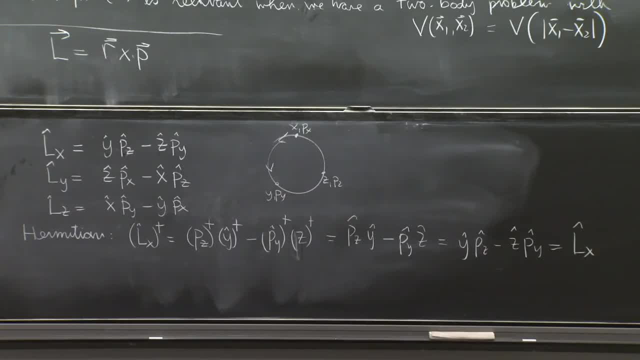 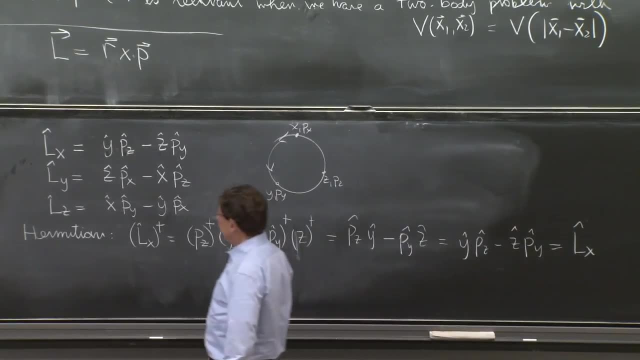 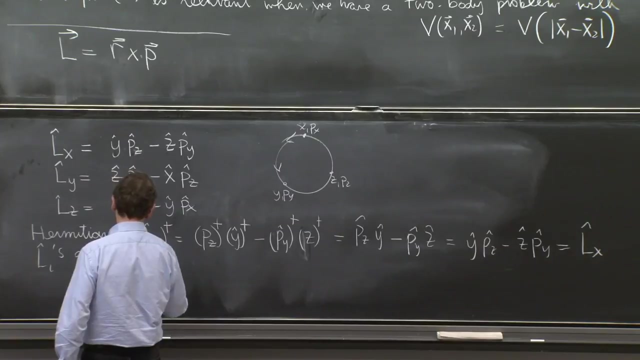 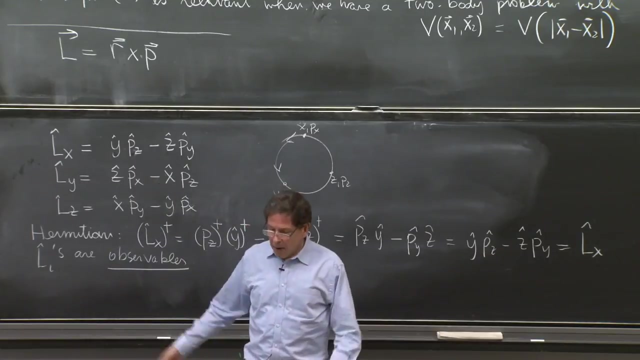 That's all you need for the operator to be an observable, And that's a very good thing. So these operators are observables, Ly's are observable, But there are other things. There are funny properties with these operators. They're not all that simple in some ways. 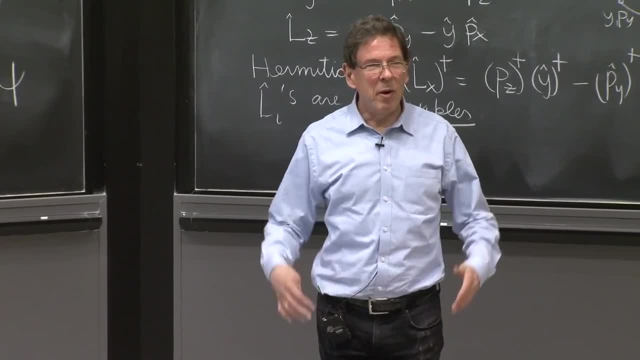 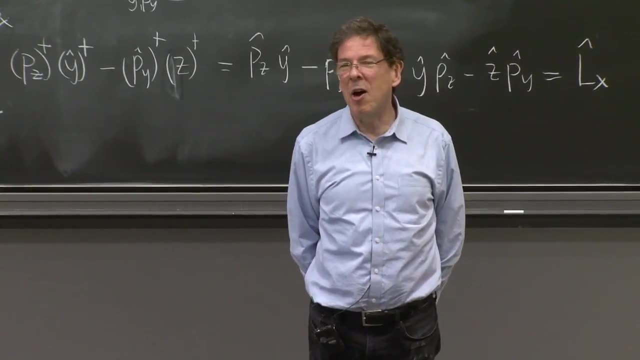 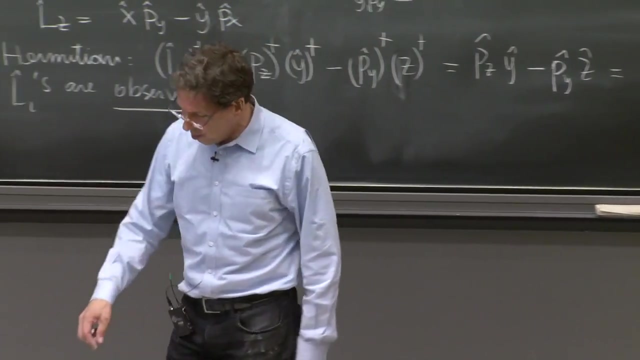 So next we have these operators. Whenever you have quantum operators, the thing you do next is compute their commutators, just like we did with x and p. We wanted to know what that commutator is. We want to know what is the commutator of this L operator. 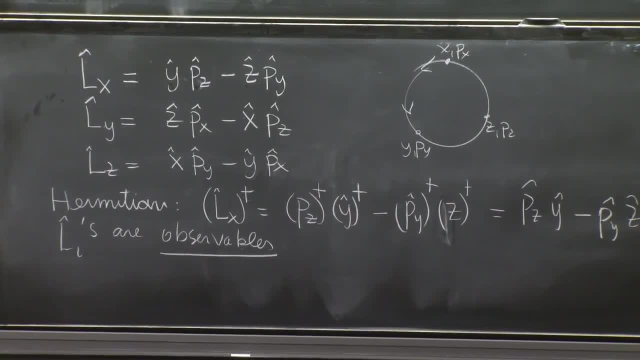 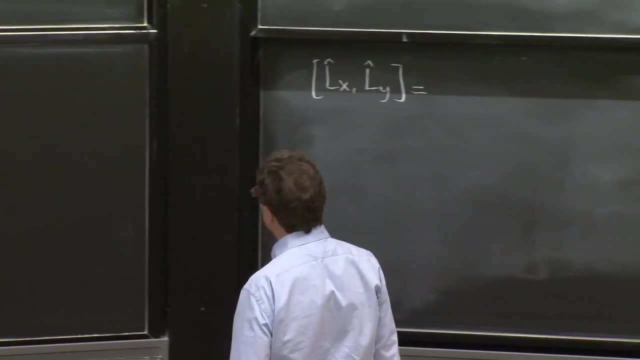 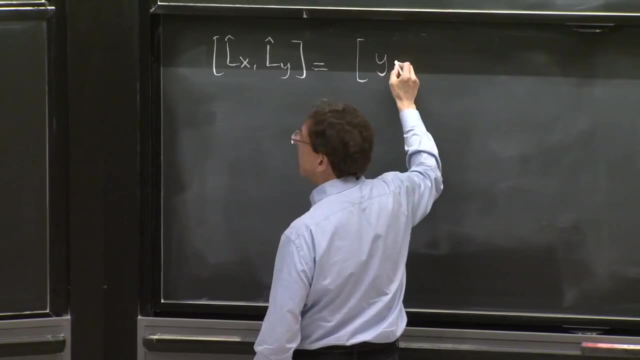 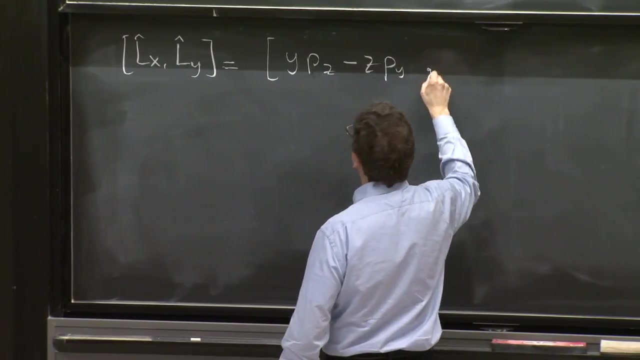 So we'll do Lx with Ly. Try to compute the commutator, So Lx is ypz. Let me forget the hats, for simplicity Minus zpy. And Ly is zpx minus Zpx, Zpx, Zpx. 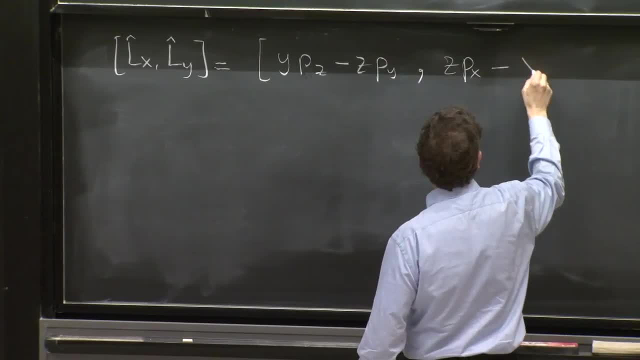 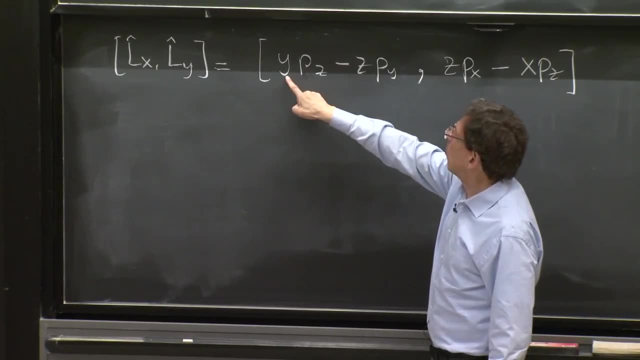 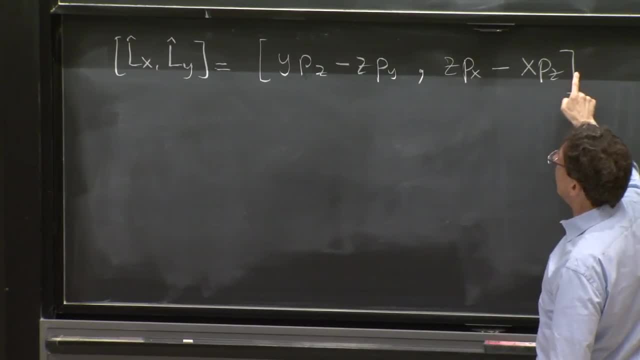 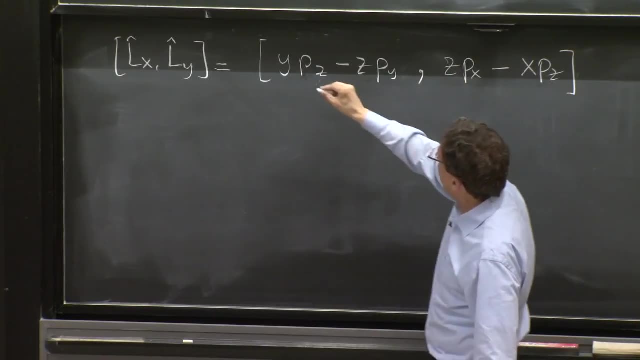 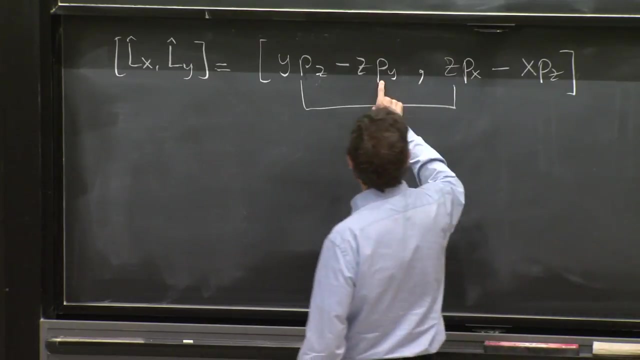 The y commutes with everything here. So the y doesn't get The pz gets stuck with the z and doesn't care about this. So this term just talks to that term And here the zpy, the py doesn't care about anybody here. 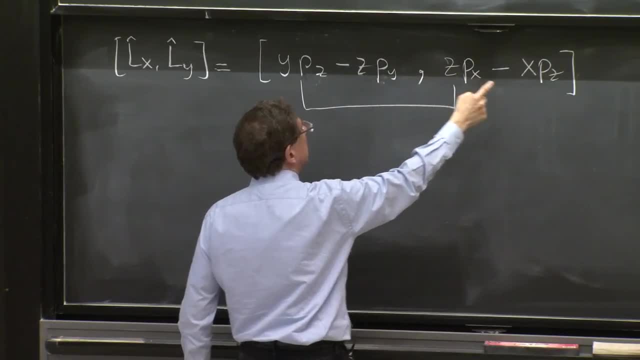 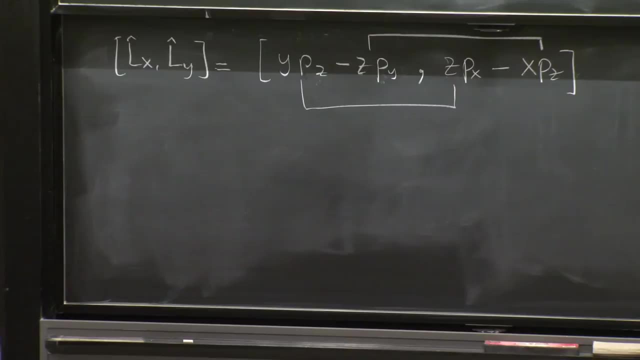 But the z? well, it doesn't care about that z, but it does care about this Pz, So the only contribution. there could have been four terms out of this commutator, but only two are relevant, So let's write them down. 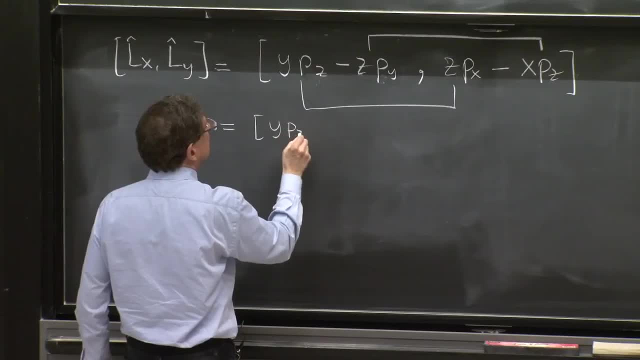 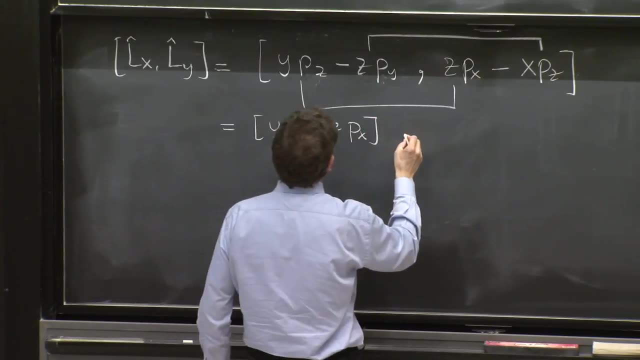 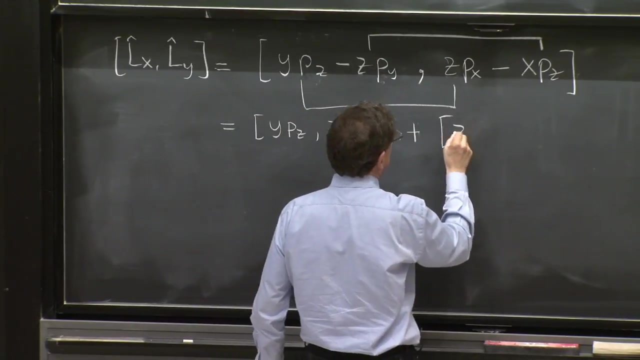 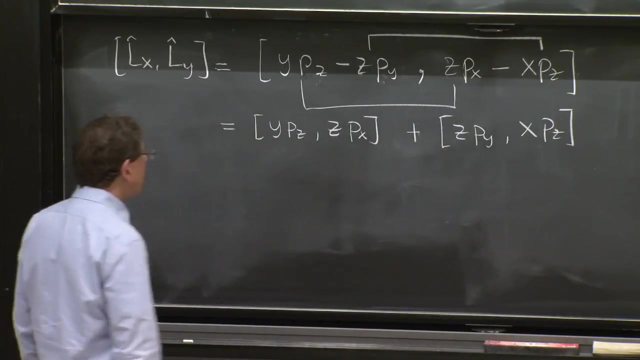 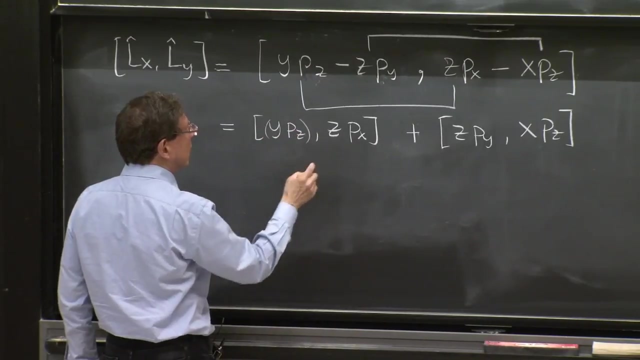 yPz with zPx minus and minus it's a plus zPy- xPz. Well, you can start peeling off things You can think of. This is a single operator with this too, And it will fail to commute with the first. 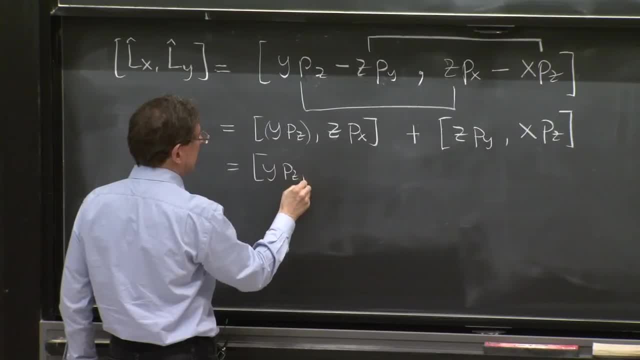 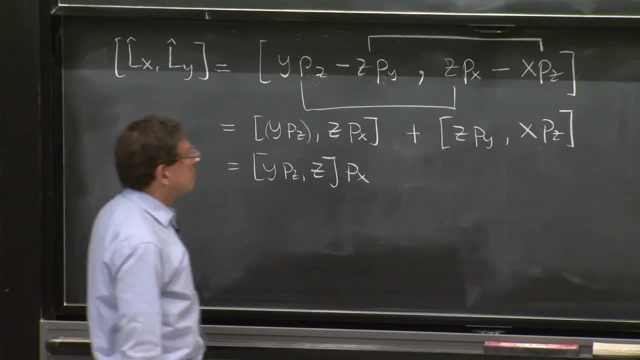 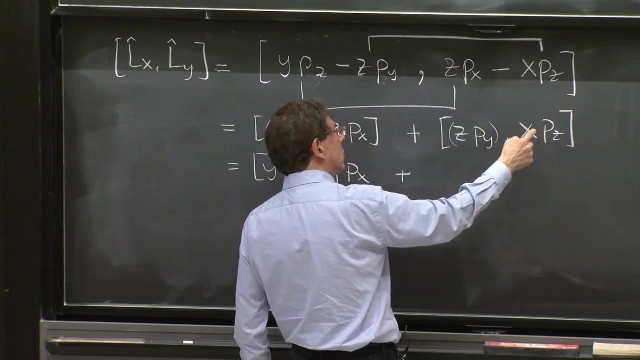 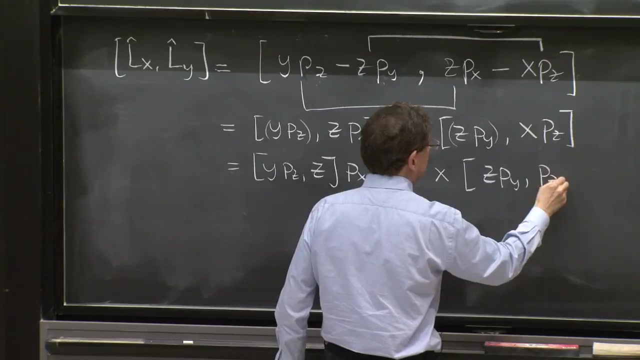 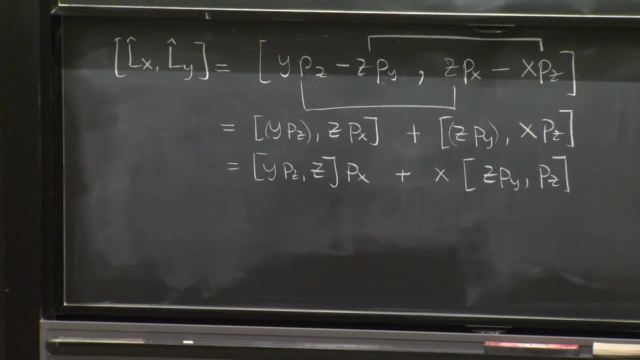 So you have yPz, zPx. That's all this commutator gives. And the same thing here. This fails to commute, just with Pz. So the x can go out, xzPy, And then here the y actually can go out. 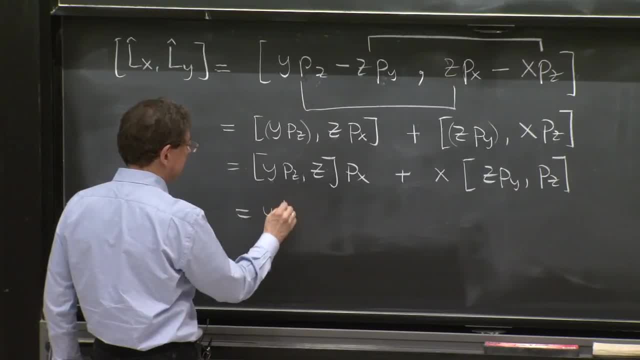 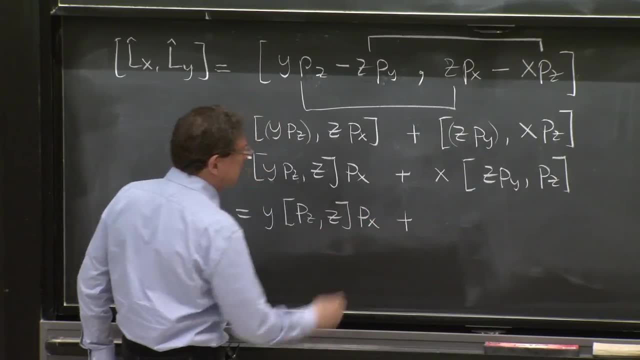 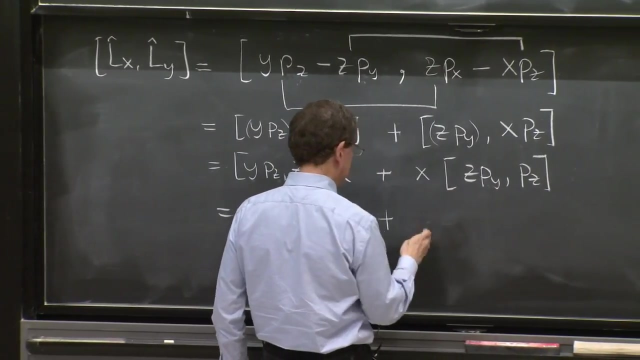 Doesn't care about the z Goes out on the left. Not that it matters much here, but that's how using the commutator identities does And this, This, This, This And this Py can go out. It must go out on the right. 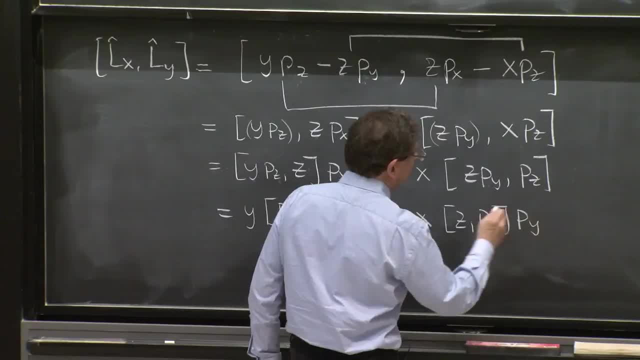 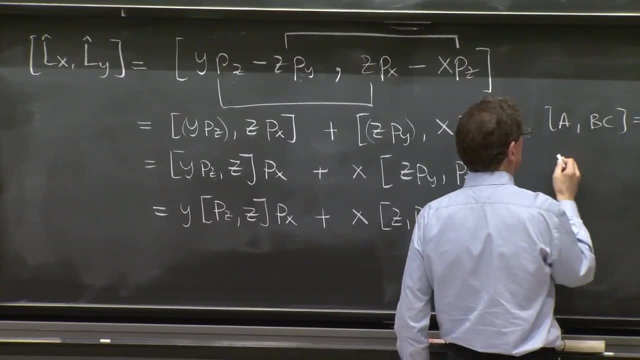 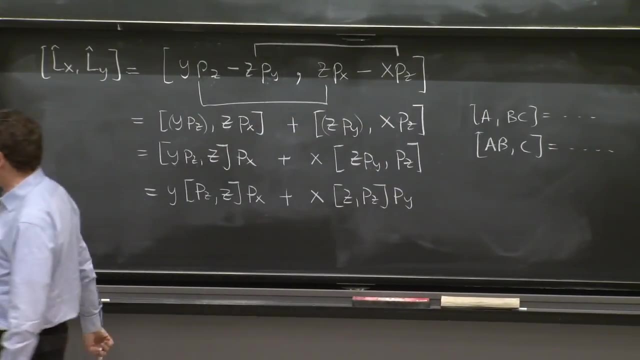 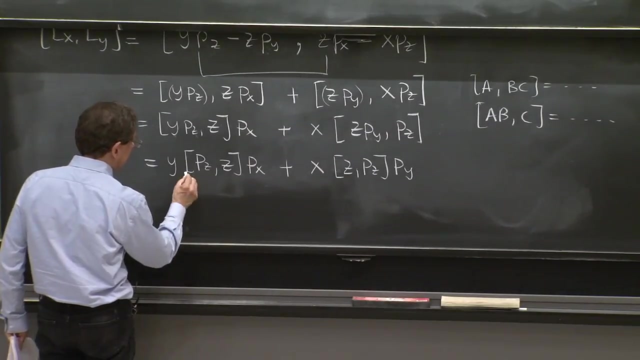 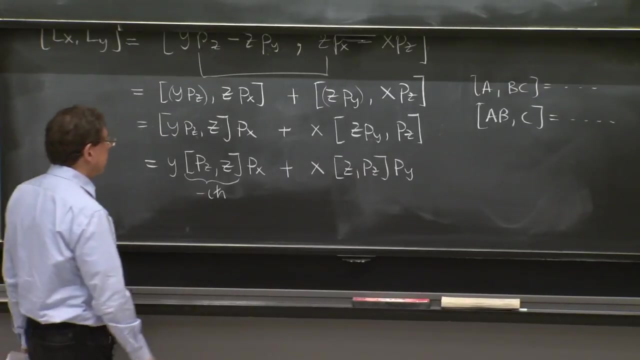 zPz. I'm basing this on this identity, which you have a b c commutator and then a b c commutators, how things distribute. Now This is minus ih bar And this is ih bar. 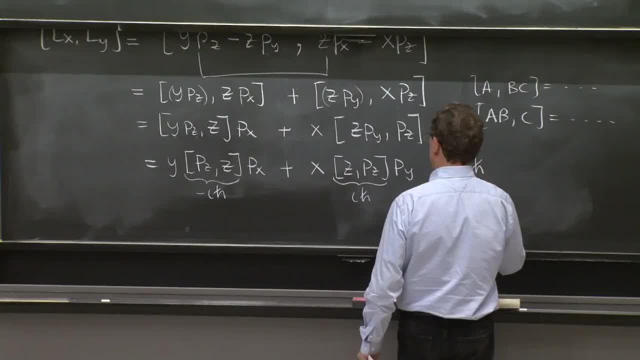 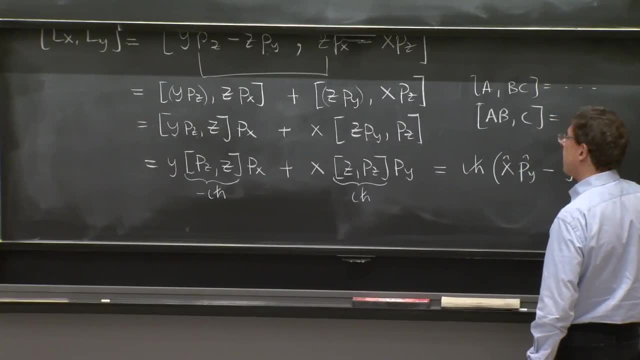 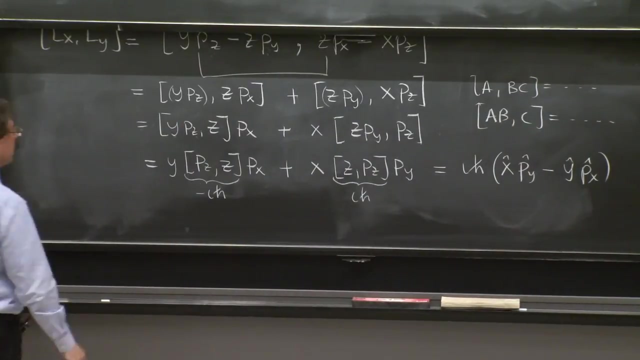 So here we get ih bar, xPy minus yPx. See, Everything came out in the right place And this is minus ih bar, This is minus yPx, This is minus yPx, This is minus yPx position, and you recognize that operator as Lz. 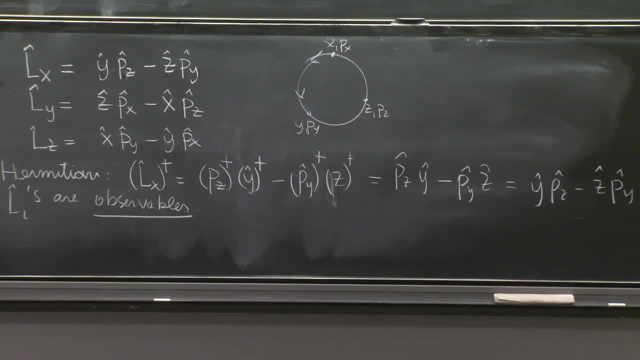 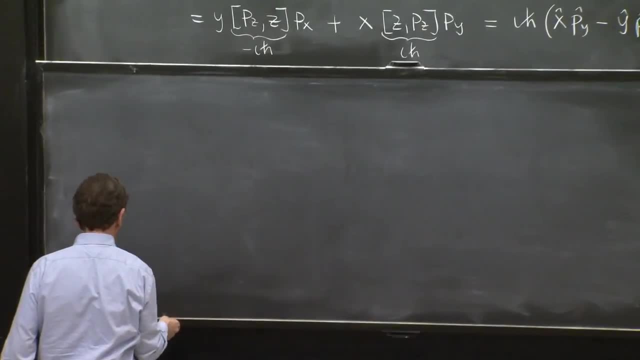 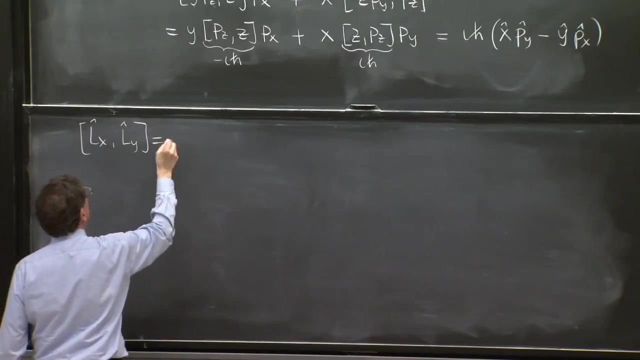 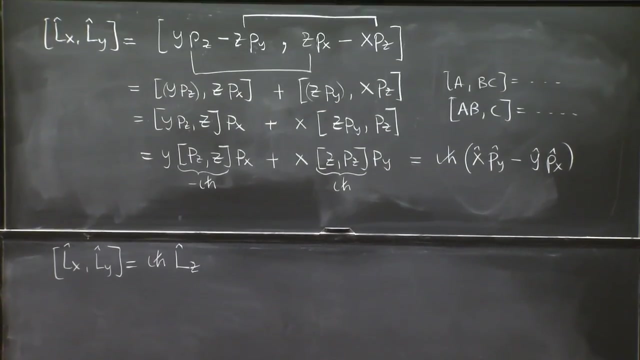 So this commutator here has given you Lx with Ly, equal ih bar Lz. It's a very interesting and fascinating property that somehow you were doing this commutator. it could have been a mess, But it combined to give you another angular momentum. 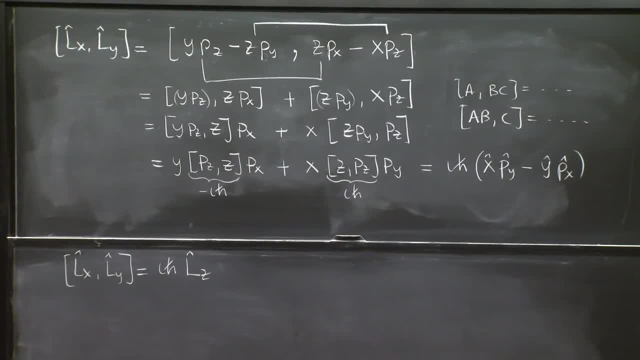 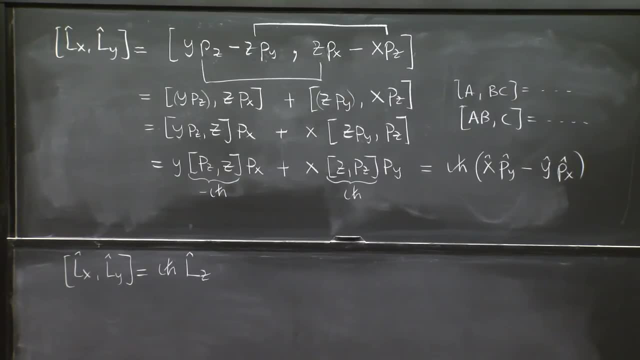 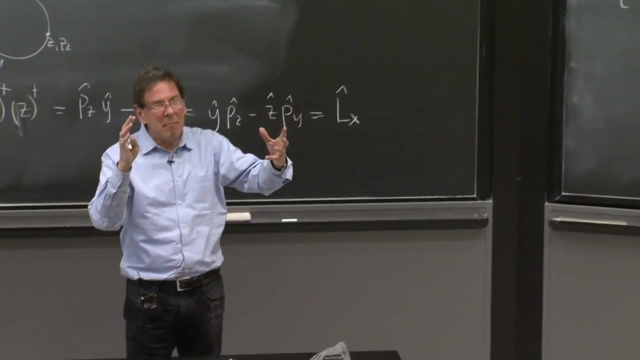 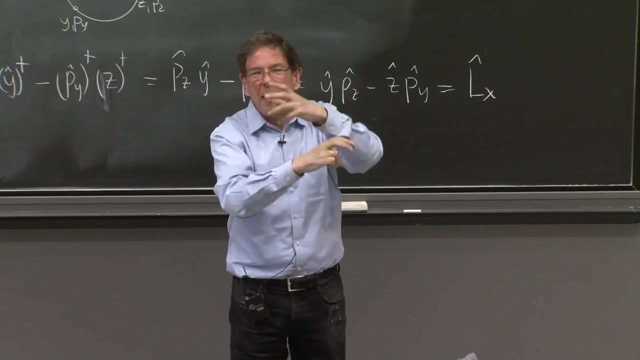 operator. Now it looks like a miracle, but physically it's not that miraculous. It actually has to do with the concept of symmetry, Symmetry transformations. if you have a symmetry transformation and you do commutators between those symmetry operators, you must get an operator that corresponds to that symmetry. 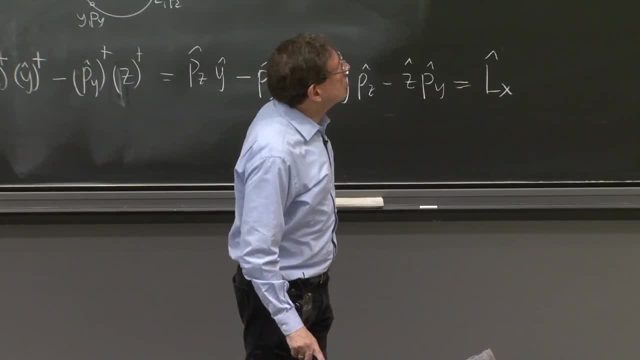 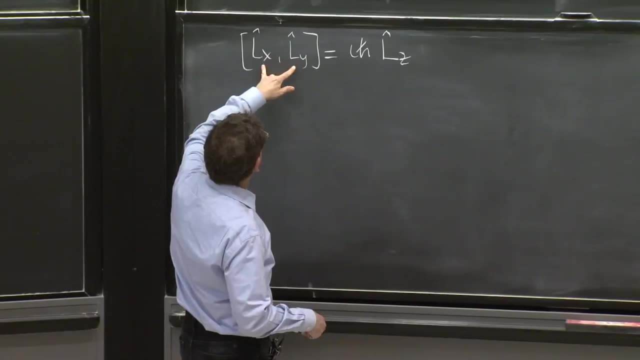 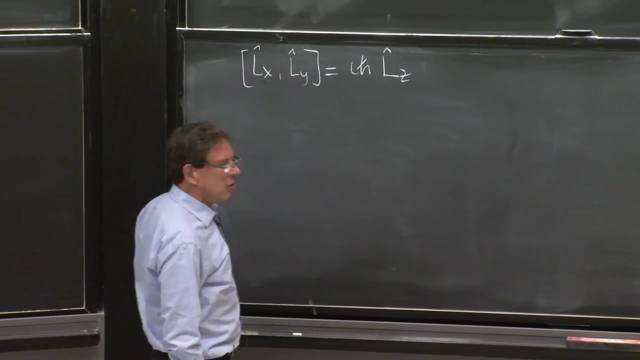 Or you must get a symmetry at the very least. So if we say that the potential has spherical symmetry, that suggests that when you do operations with these operators that generate rotations, you should get some rotation here, And alternatively- although again this is suggestive- 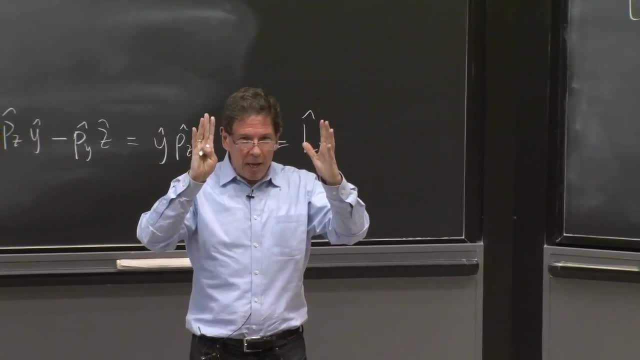 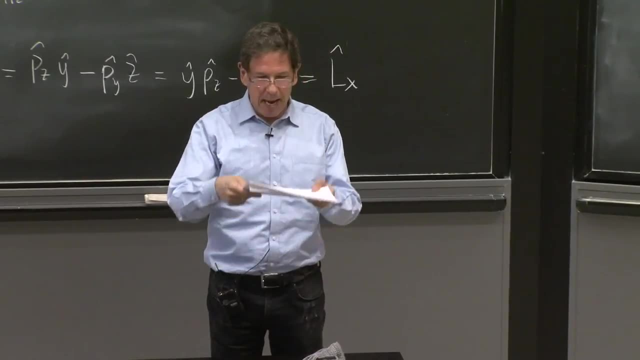 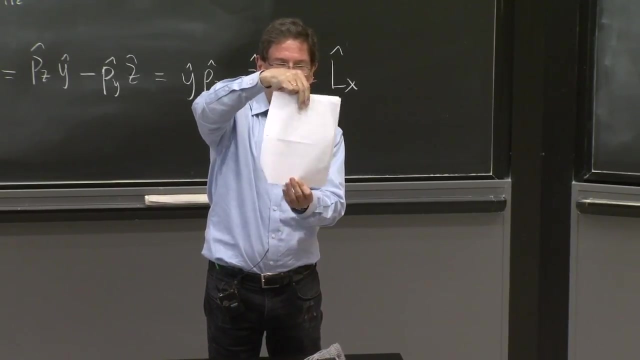 it can be made very precise. when you do rotations in different order, you don't get the same thing at the end. Everybody knows if you have a page and you do one rotation and then the other, as opposed to the other, and then the first one. 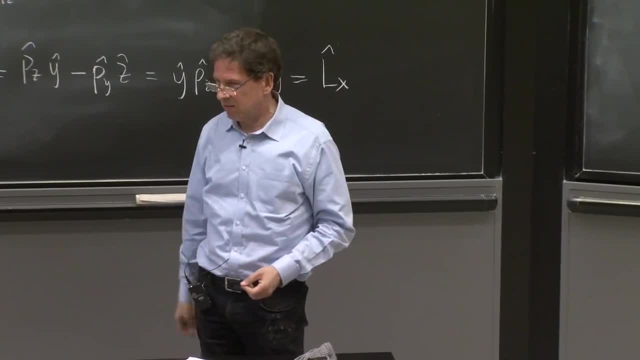 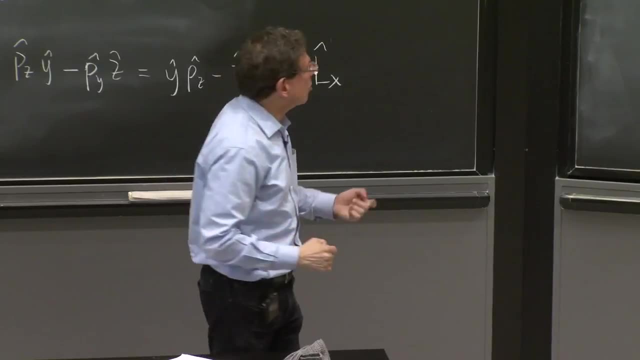 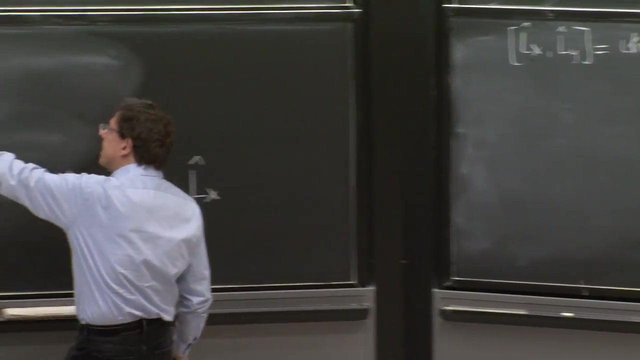 you don't get the same thing. Rotations do not. Rotations do not commute. A single rotation does commute in one direction, but rotations in different directions don't commute. That is the reason for this equation And this equation: as we said, everything is cyclic. 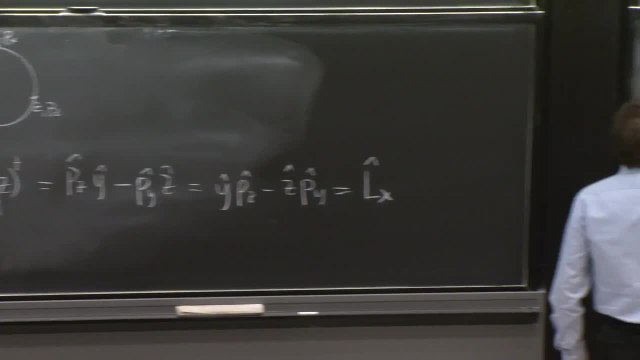 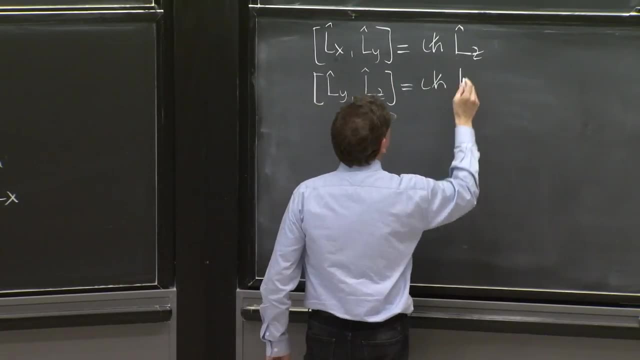 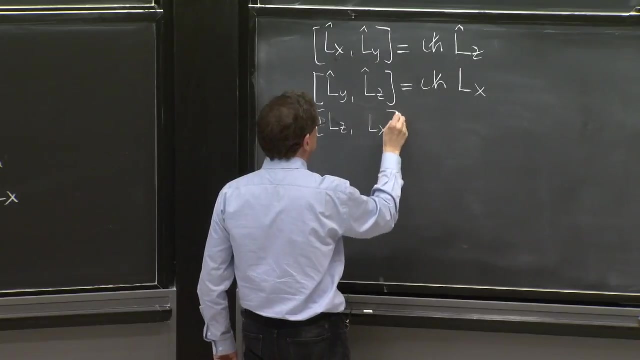 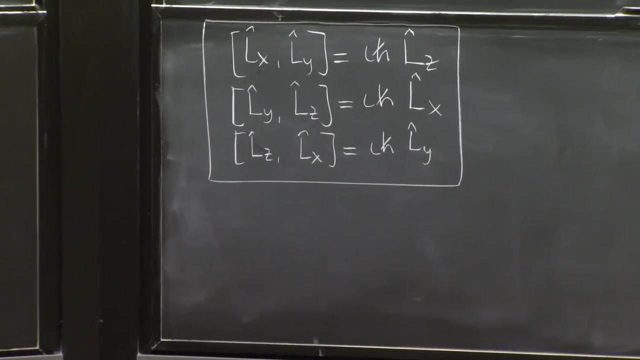 So you don't have to work again to argue that then Ly Lz going cyclic must be equal to ih bar Lx, And that Lz Lx must be ih bar Ly, And this is called the quantum algebra of angular momentum. 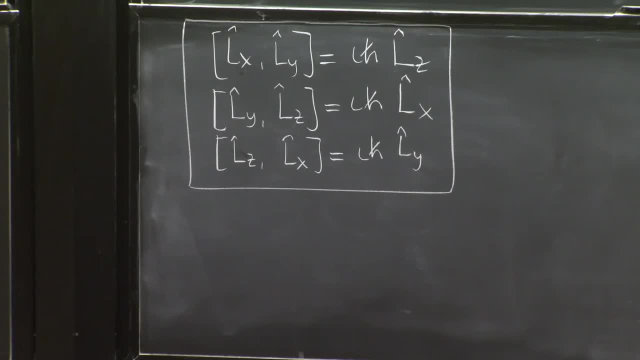 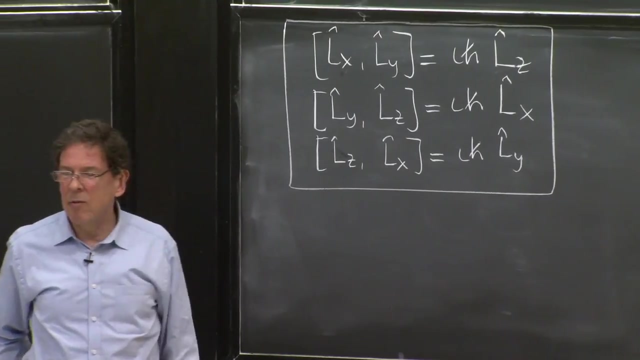 In fact it is so important that this algebra appears in all fields. It appears in all fields of physics and mathematics And all kinds of things show up. This algebra is related to the algebra of generators of the group SU2, special unitary transformations. 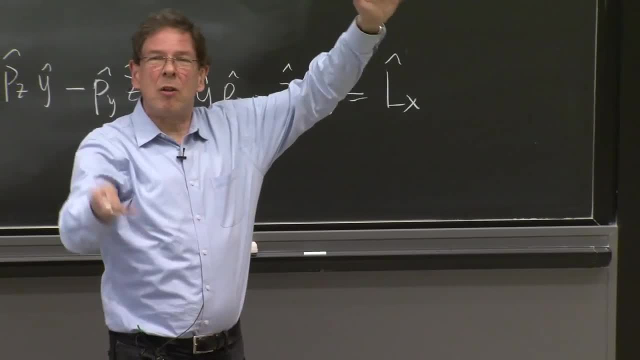 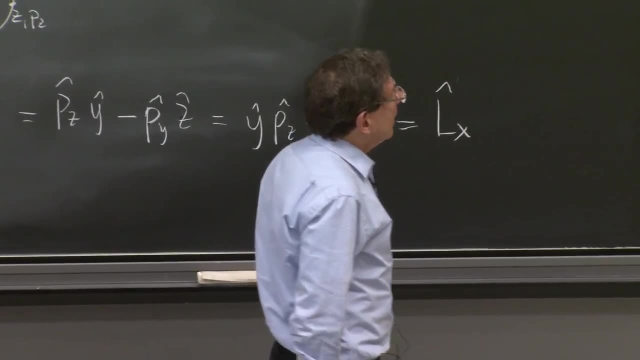 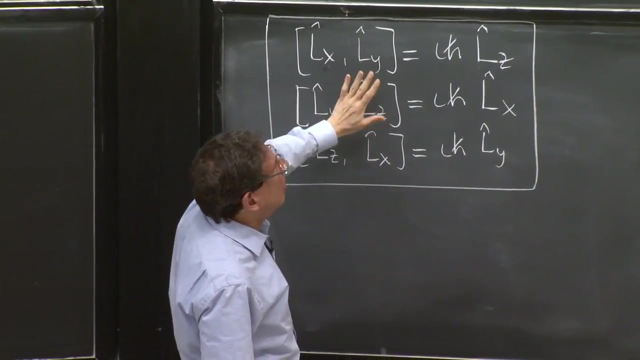 in two dimensions. It is related to the orthogonal group in three dimensions where you rotate things in three-dimensional space. It is related to the orthogonal group in three dimensions. It is here the algebra of operators And in a sense it's a deeper result than the derivation. 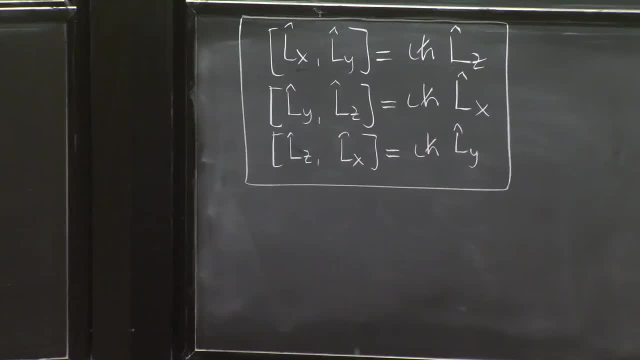 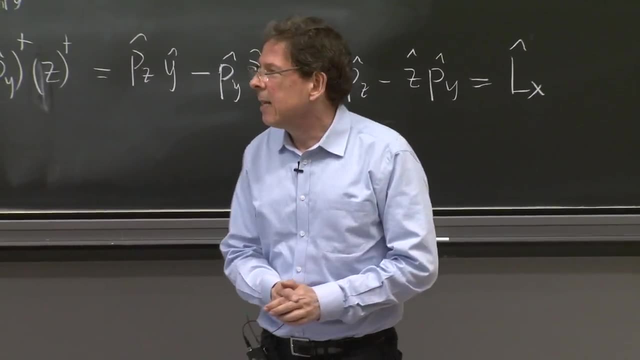 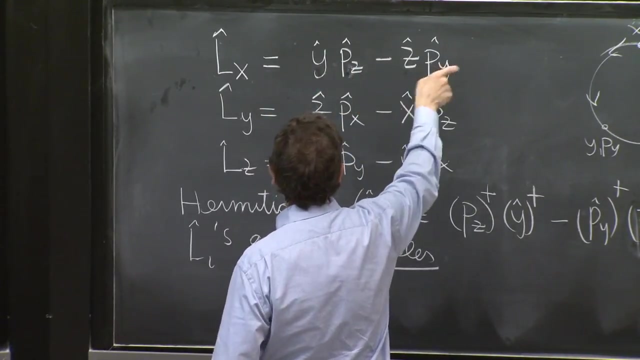 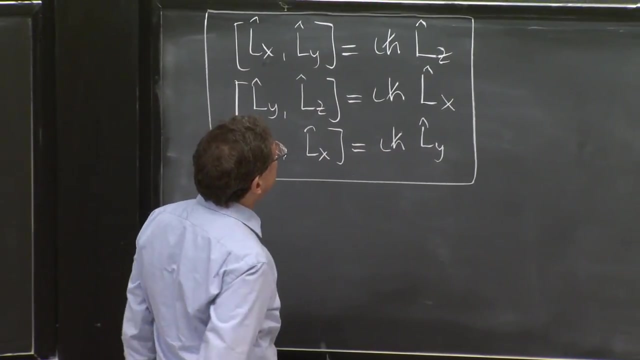 It is one of those cases when you start with something very concrete and you suddenly discover a structure that is rather universal, Because we started with very concrete representation of l's in terms of yp's and all these things Right, But then they form a consistent unit by themselves.